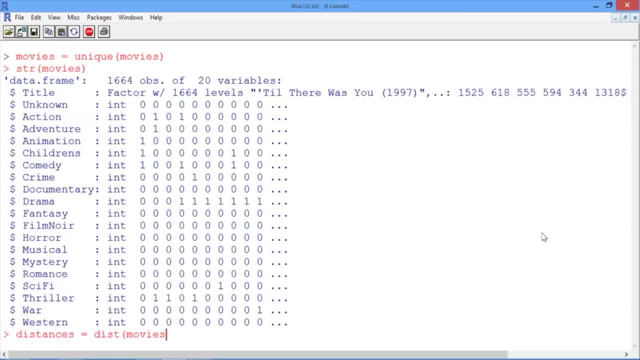 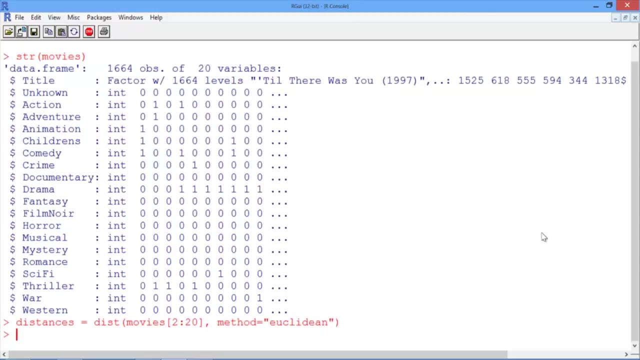 and we'll use the dist function, where the first argument is movies- this is what we want to cluster on, And the second argument is method equals in quotes Euclidean, meaning that we want to use Euclidean distance. Now let's cluster our movies using the hclust function for hierarchical. 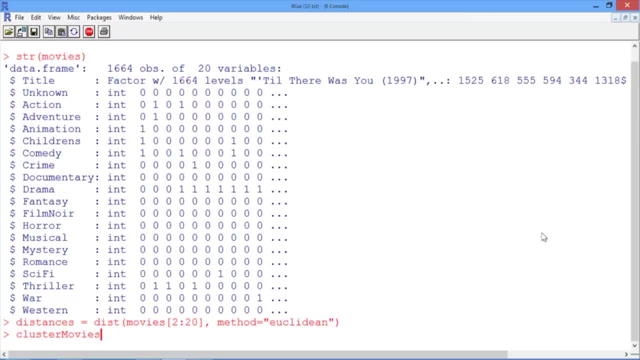 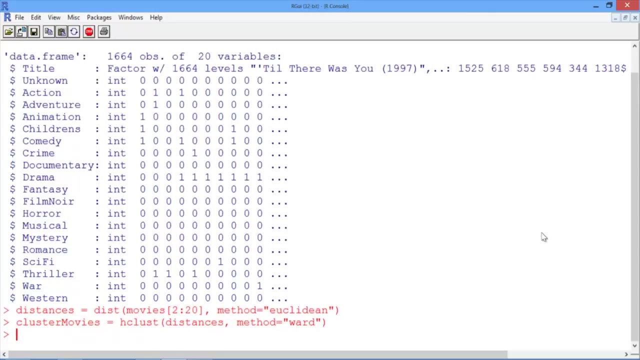 clustering. We'll call the output cluster movies and use hclust, where the first argument is distances- the output of the dist function- and the second argument is method equals ward. The ward method cares about the distance between clusters using centroid distance. 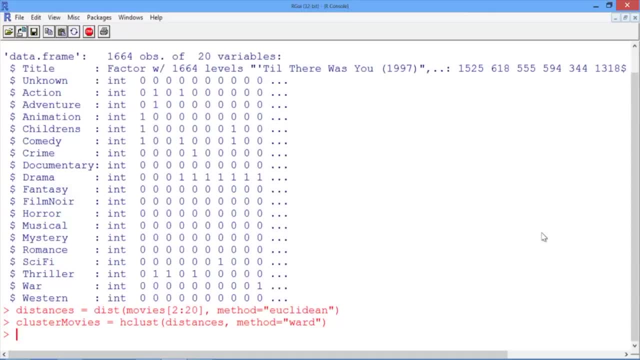 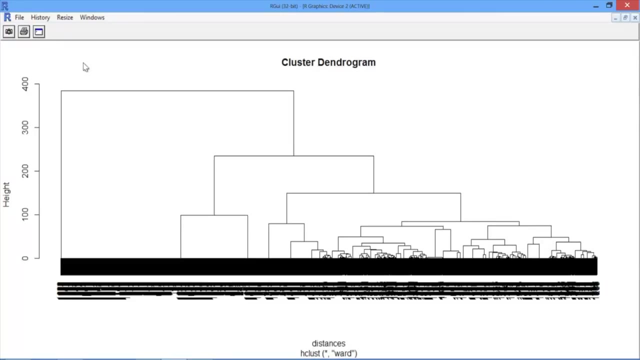 and also the variance in each of the clusters. Now let's plot the dendrogram of our clustering algorithm by typing plot and then, in parentheses, cluster movies. This dendrogram might look a little strange. We have all this black along the bottom, Remember. 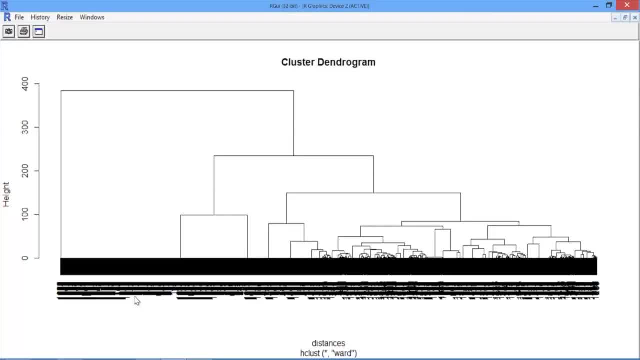 that dendrogram lists all of the data points along the bottom, But when there are over a thousand data points it's impossible to read. We'll see later how to assign our clusters to groups so that we can analyze which data points are in which cluster. 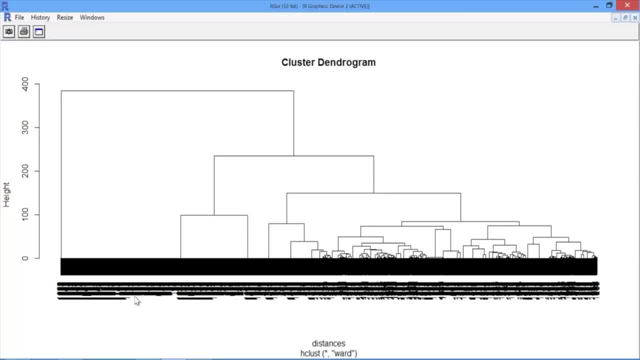 So, looking at this dendrogram, how many clusters would you pick? It looks like maybe three or four clusters would be a good choice according to the dendrogram, but let's keep our application in mind too. We probably want more than two, three or even four clusters of movies to make recommendations. 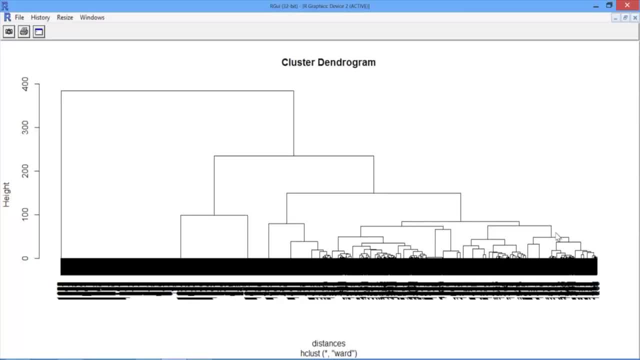 to users. It looks like there's a nice spot down here where there's ten clusters. This is probably better for our application. We could select even more clusters if we want to have very specific genre groups. If you want a lot of clusters, it's hard to pick. 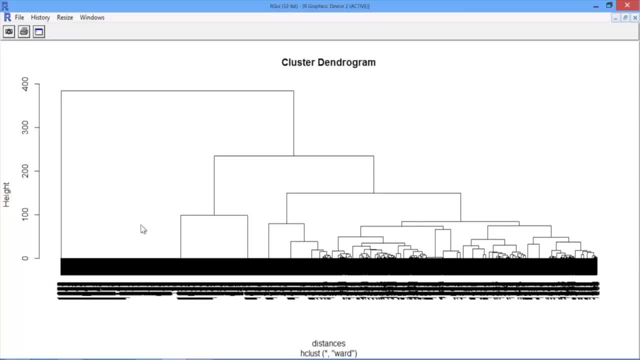 the right number from the dendrogram. You need to use your understanding of the problem to pick the number of clusters. Let's stick with 10 clusters for now, combining what we learned from the dendrogram with our understanding of the problem. Now, back in our R console, we can label each of the data points according to what cluster. 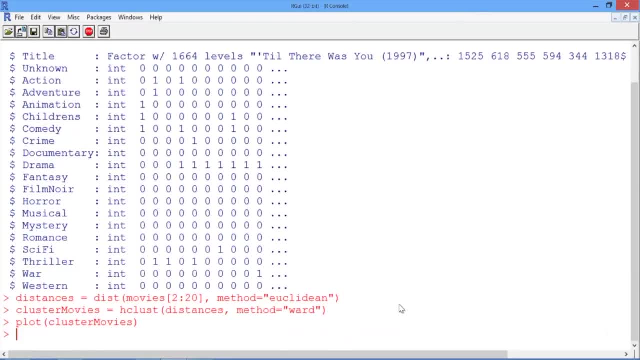 it belongs to using the cuTree function. So let's type cluster groups equals cuTree, and then in parentheses the name of the cluster. So let's type cluster groups equals cuTree, and then in parentheses the name of the cluster. So that's how we can label. 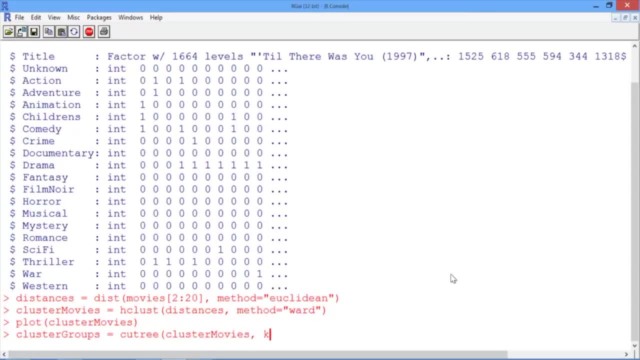 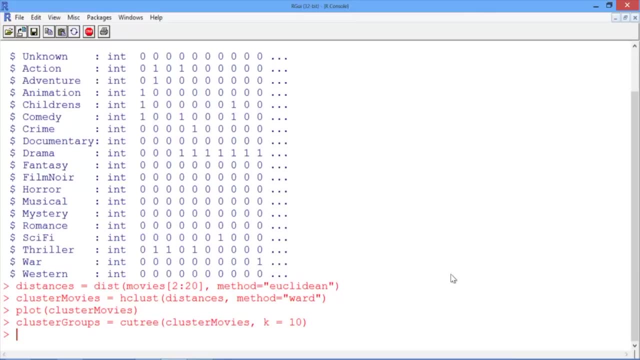 name of our clustering cluster movies, and then k equals 10,, since we selected 10 clusters. Now let's figure out what the clusters are like. We'll use the tapply function to compute the percentage of movies in each genre and cluster. 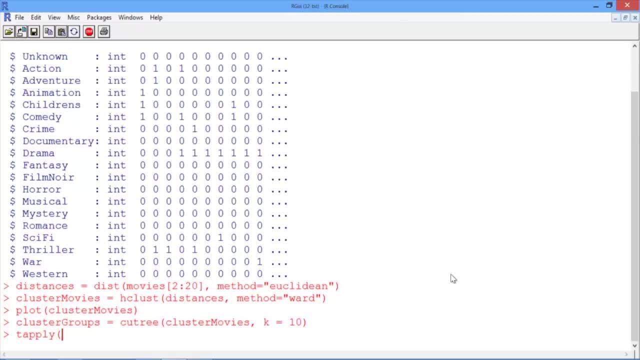 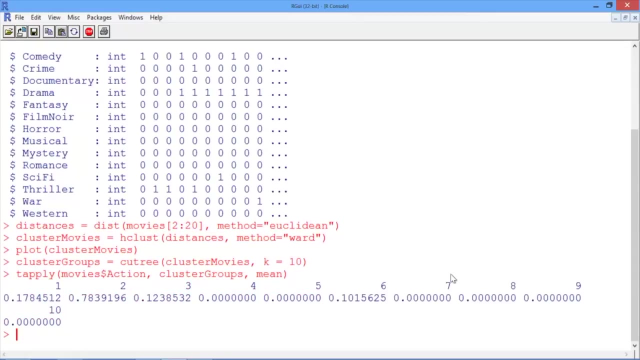 So let's type tapply and then give us the first argument: movies, dollar sign, action. we'll start with the action genre and then cluster groups and then mean: So what does this do? It divides our data points into the 10 clusters and then 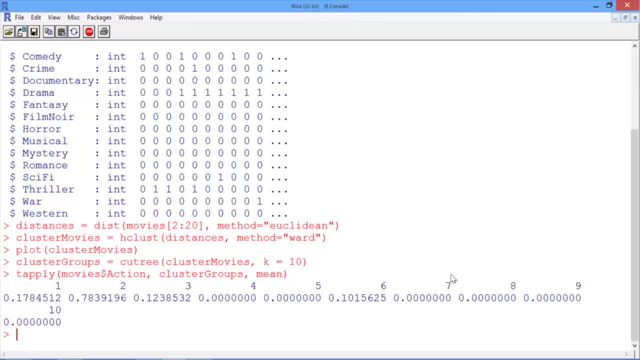 computes the average value of the action variable for each cluster. Remember that the action variable is a binary variable with value 0 or 1. So by computing the average of this variable, we're computing the percentage of movies in that cluster that belong in that genre. 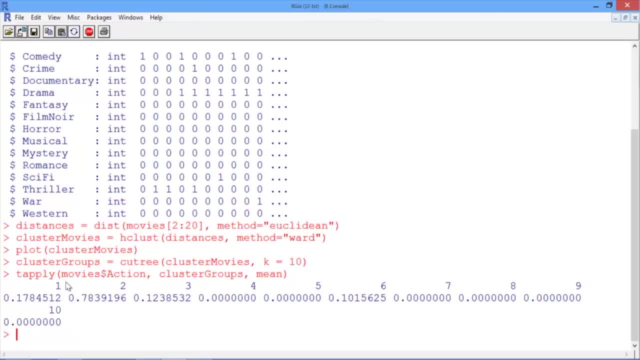 So we can see here that in cluster 2, about 78% of the movies have the action genre label, whereas in cluster 4, none of the movies are labeled as action movies. Let's try this again, but this time let's look at the. 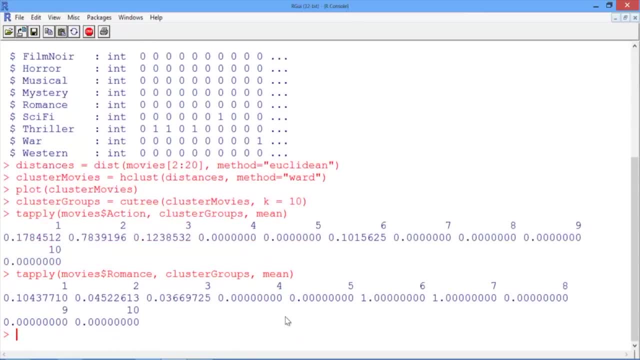 romance genre. Here we can see that all of the movies in cluster 6 are action movies. The movies in cluster 6 and 7 are labeled as romance movies, whereas only 4% of the movies in cluster 2 are labeled as romance movies. 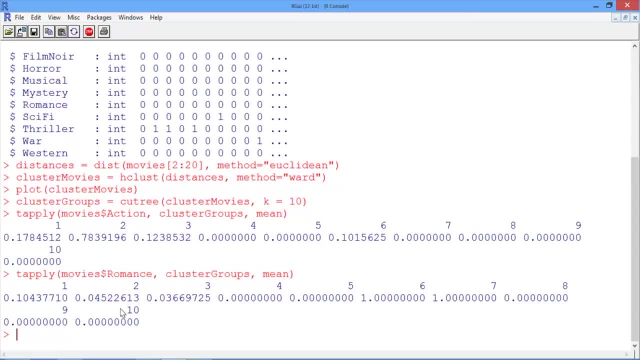 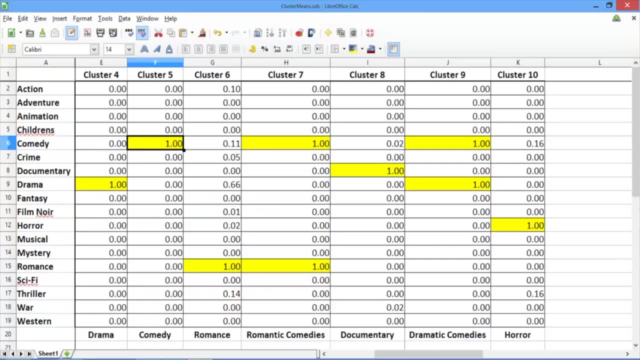 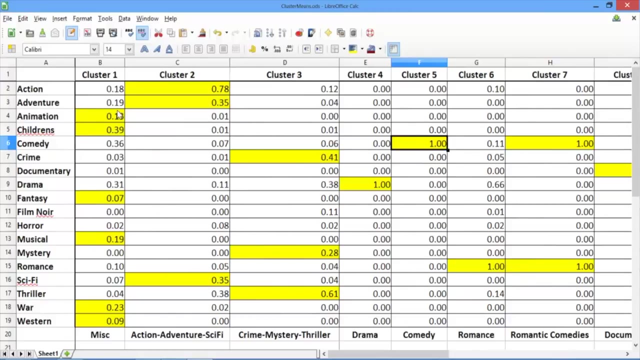 We can repeat this for each genre. If you do, you can create a large table to better analyze the clusters, which I saved to a spreadsheet. Let's take a look Here. we have in each column the cluster and in each row. 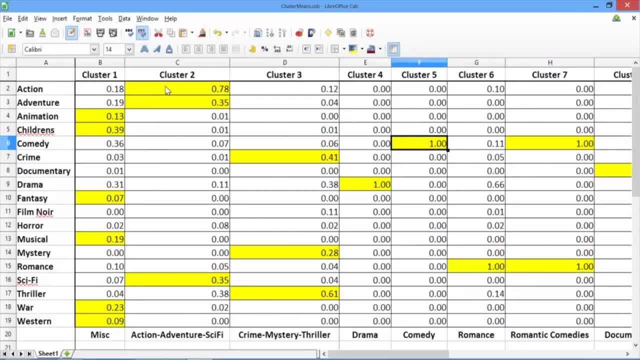 the genre. I highlighted the cells that have a higher than average value. So we can see here in cluster 2, as we saw before, that cluster 2 has a high number of action movies. Cluster 1 has a little bit of everything, some animation. 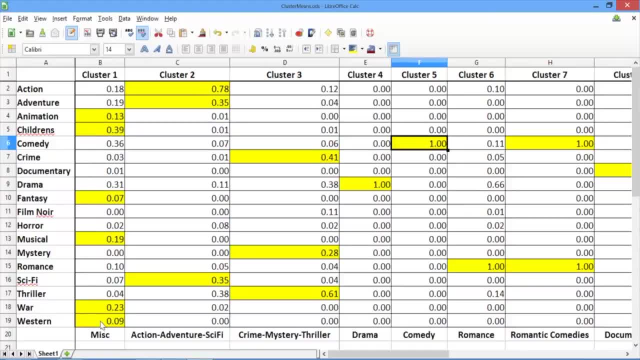 children's fantasy, musicals, war and westerns. So I'm calling this the miscellaneous cluster. Cluster 2 has a lot of the action, adventure and sci-fi movies. Cluster 3 has the crime mystery thriller movies. 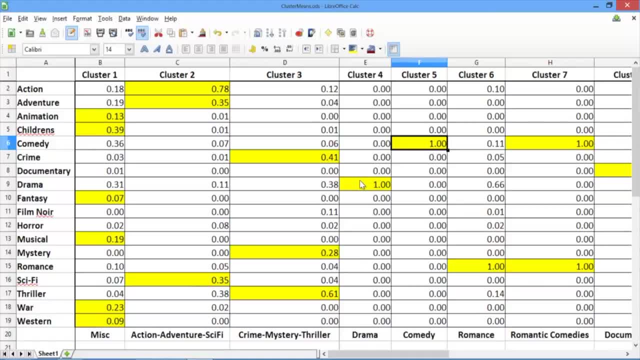 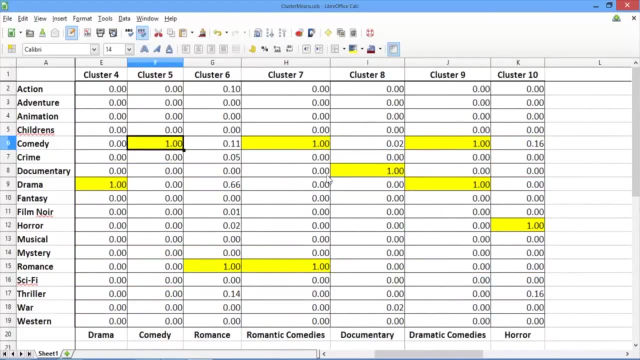 Cluster 4 exclusively has drama movies. Cluster 5 exclusively has comedies. Cluster 6 has a lot of the romance movies. Cluster 7 has movies that are comedies and romance movies, So I'm calling these the romantic comedies. Cluster 8 has the documentary movies. 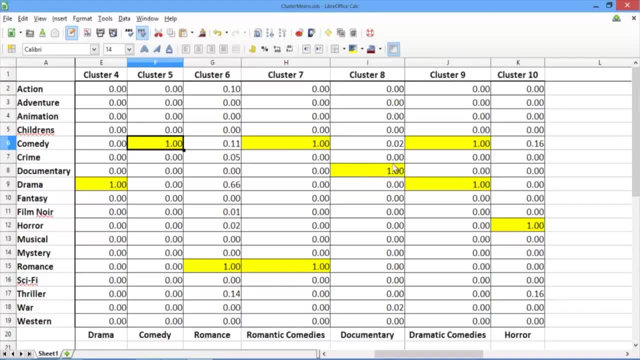 Cluster 9 has the animated movies. Cluster 10 has the feature films, movies entries. Cluster 9 has the movies that are comedies and dramas, so the dramatic comedies, And cluster 10 has the horror flicks. Knowing common movie genres, these clusters- 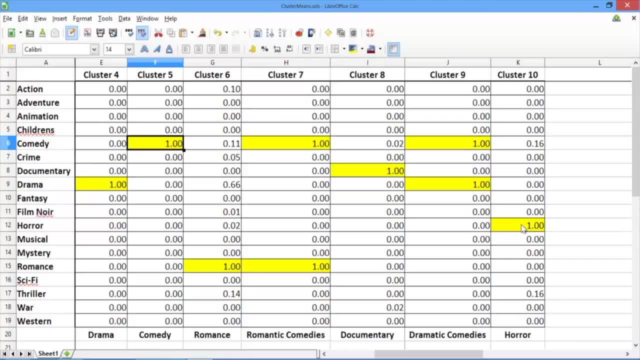 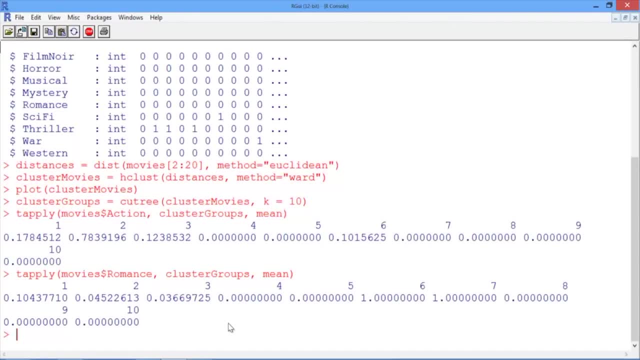 seem to make a lot of sense. So now back in our R console. let's see how these clusters could be used in a recommendation system. Remember that Amy liked the movie Men in Black. Let's figure out what cluster Men in Black is in. 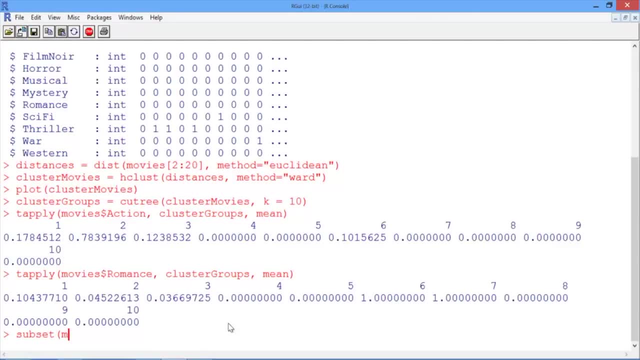 We'll use the subset function to take a subset of movies and only look at the movies where the title is equal to Men in Black, and then parentheses: 1997.. Close the quotes in the parentheses. I knew that this is the title of Men in Black. 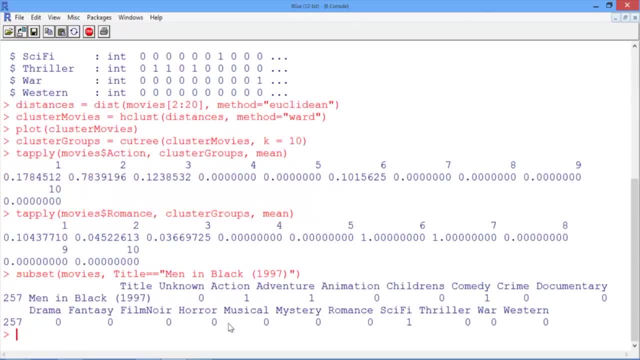 because I looked it up in our data set. So what looks like Men in Black is the 257th row in our data. So which cluster did the 257th movie go into? We can figure this out by typing cluster groups and then. 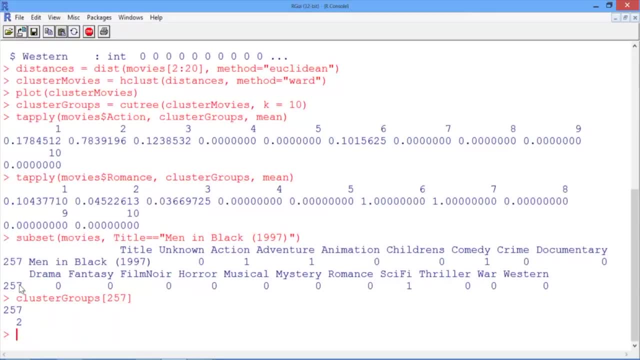 square brackets: 257.. It looks like Men in Black went into cluster 2.. That makes sense, since we just saw that cluster 2 is the Action Adventure Sci-Fi cluster. So let's create a new data set with just the movies from cluster 2.. 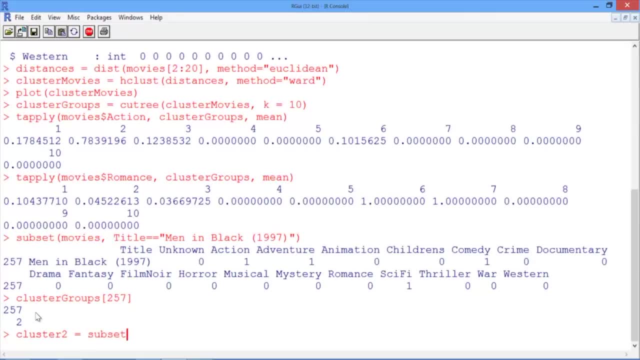 We'll call it Action Adventure Sci-Fi. We'll call it Action Adventure Sci-Fi. We'll call it Action Adventure Sci-Fi. We'll call it cluster 2 and use the subset function to take a subset of movies. only taking the observations for which cluster groups is equal to 2..